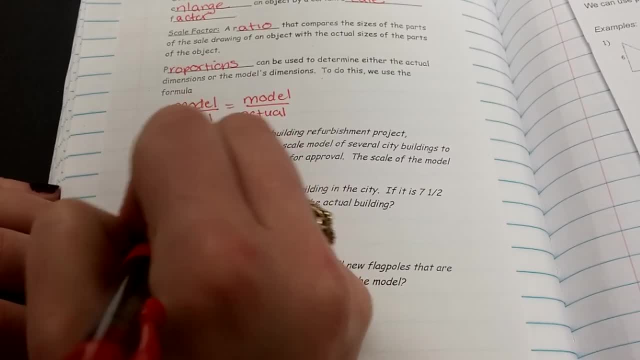 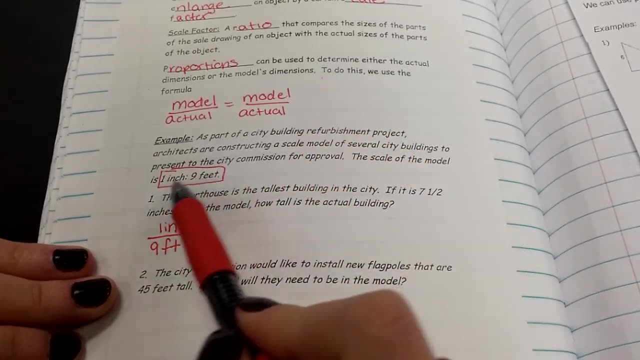 fraction. in my proportion, 1 inch in the model is to 9 feet. So in sixth grade you learned about there's three ways to write ratios. You can write them with a colon, you can write them with the word two or you can write them as a fraction. 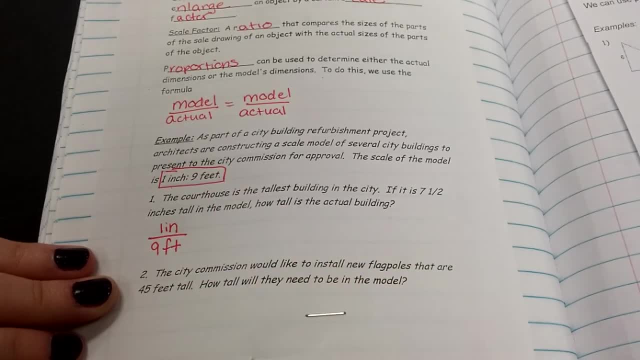 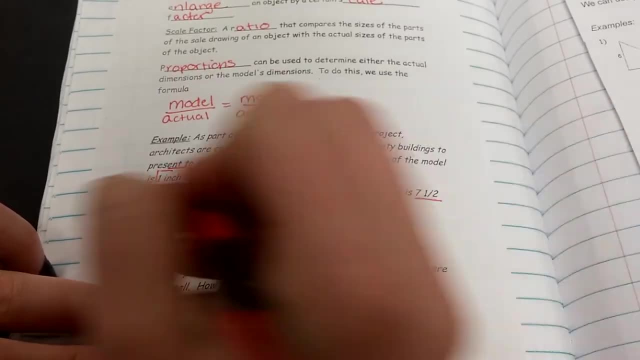 So we're taking this one- It's a proportion that's written with a colon- and we're changing it into a proportion written with a fraction, or a ratio written with a fraction That's equal to 7 and a half inches tall. So again we can match the units just like. 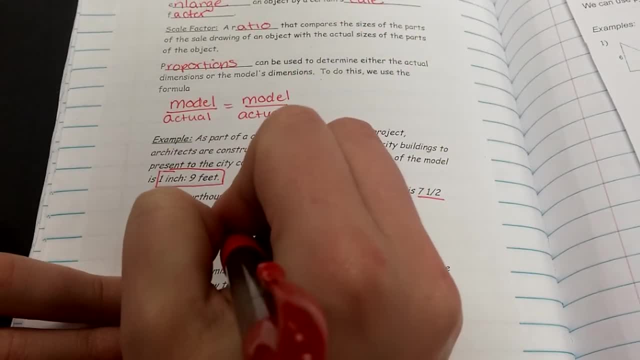 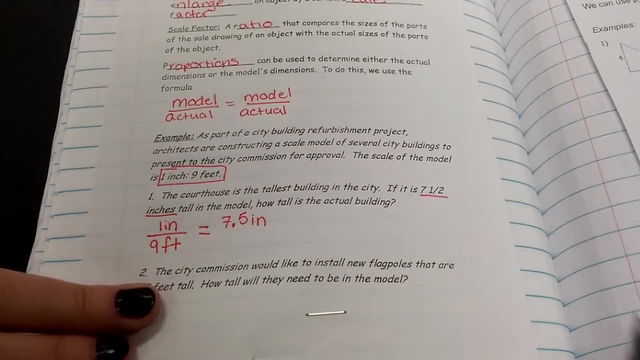 we did with the word problem. So 7 and a half inches- And in this case it would be okay to change 7 and a half with the fraction into 7.5 inches, It makes the math a little bit easier- Is equal to how tall is the actual building. We don't know how tall the real building is. 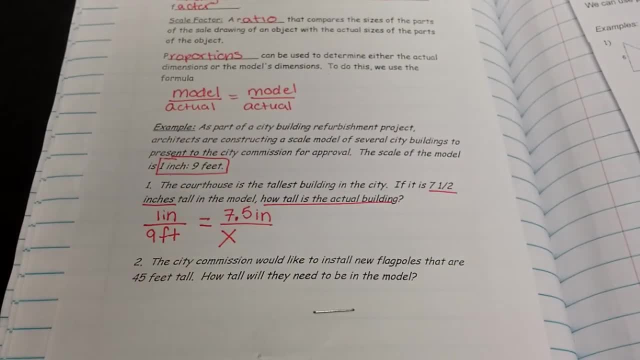 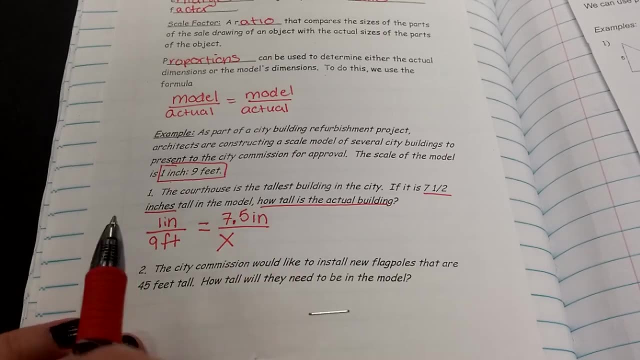 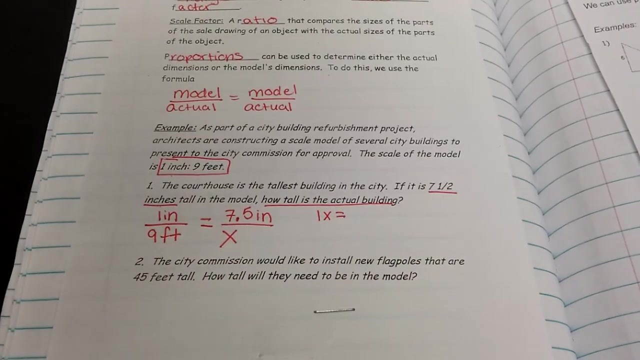 So we're going to replace the quantity that we don't know with an X. grab my calculator really quick And then we need that. then we just cross multiply to solve. So we have 1 inch times X. So 1X is equal to 9 times 7.5.. So 9 times 7.5 gives me 67.5.. And then I would 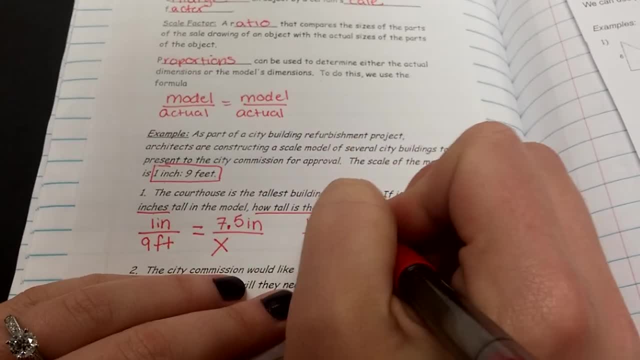 solve the proportion One times X, We would divide both sides by one And we end up with X is equal to – of X can be shifted here, though, if I forget the named expression from here, We're going to set this square cell here. Abraham would have to do it. and two, two Đây. 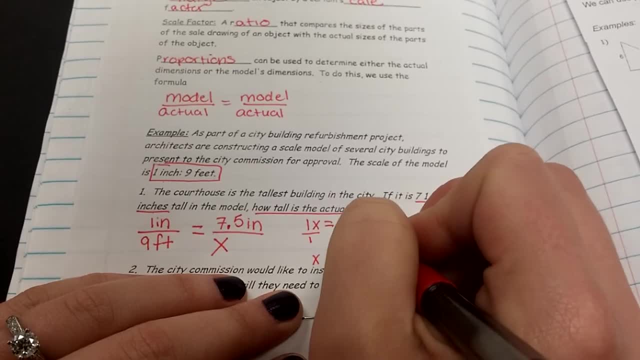 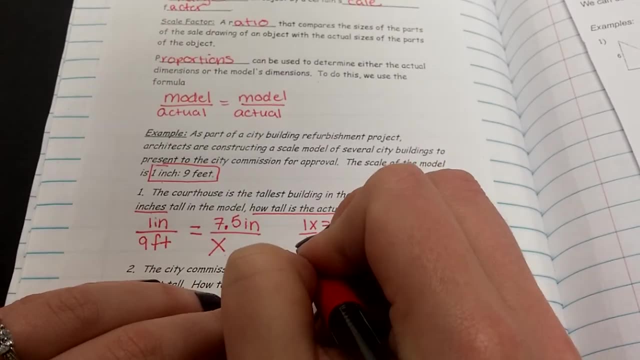 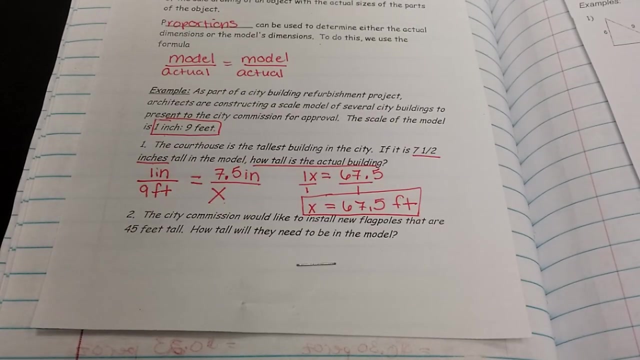 ää equal to 67.5, and we're looking for the actual dimensions, so that would be feet. example number two: the City Commission would like to install new flagpoles that are 45 feet tall. how tall they need to be in the model? so again, we go back to. 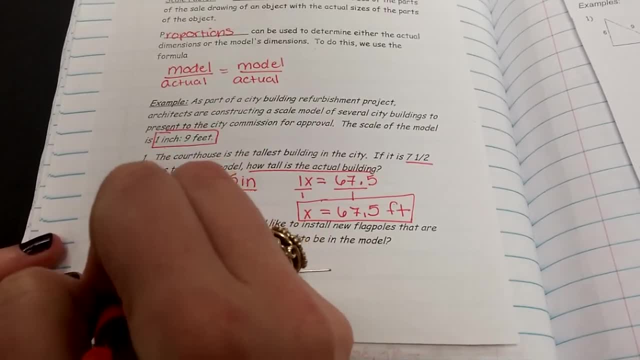 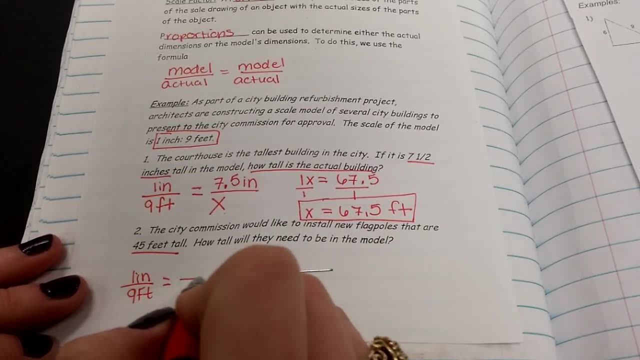 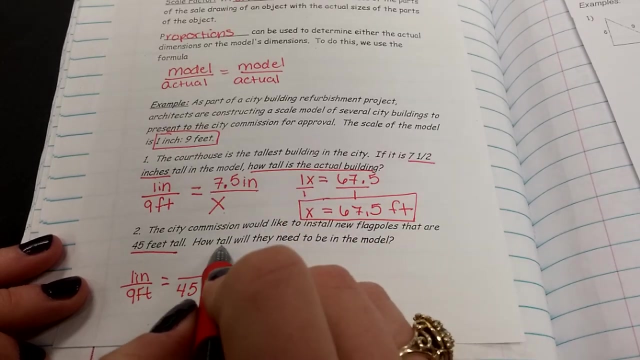 the scale factor. one inch is to nine feet. it's equal to in real life. the flagpoles are 45 feet tall, so we put that quantity in the denominator. that's an actual value, it's a real-life value and we want to know how tall will they?